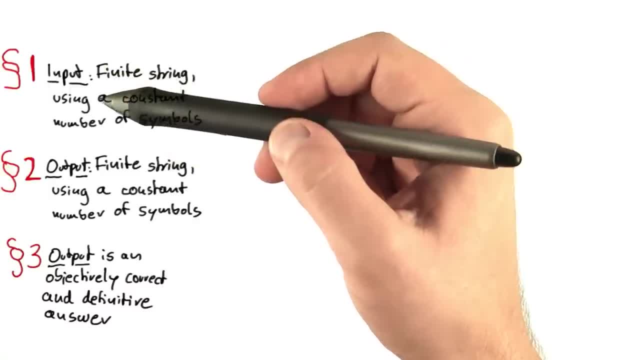 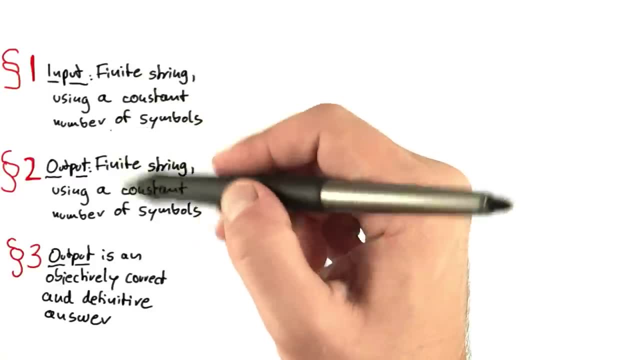 So can a computer solve any problem that meets these three requirements? And it seems in a way like a computer should be able to do that, doesn't it? I mean, the input is fit for a computer, the output is fit for a computer. We have even been very, very nitpicky with finite strings. 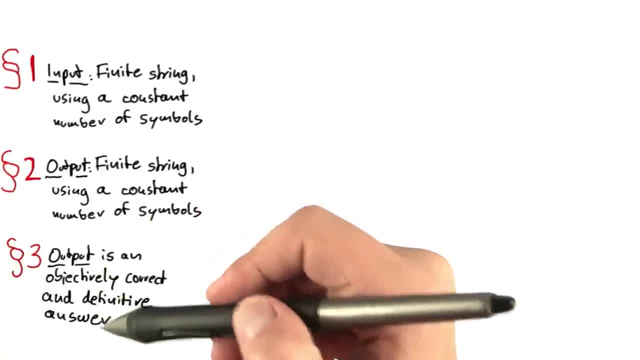 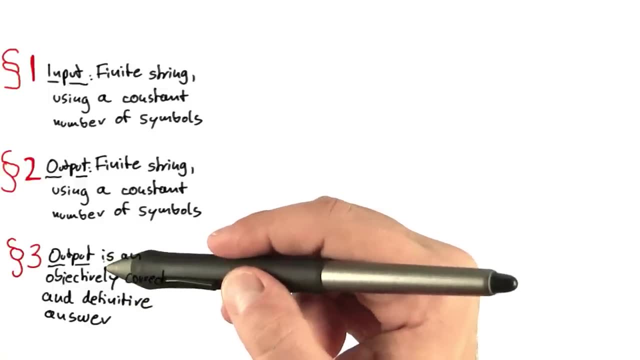 constant number of symbols, and we want an objectively correct and definitive answer. No grading students' essays. no predicting the future. no looking at pictures and telling us if they're beautiful. I'm now going to show you a problem that meets these three criteria. I will 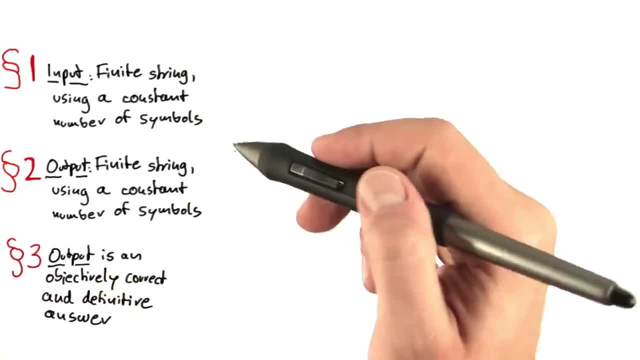 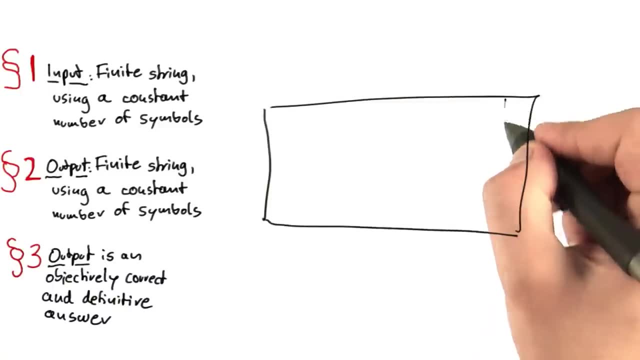 also be able to show you that no computer can ever solve it, And this is actually a problem where it would be very useful to have a computer being able to solve it. So I guess you've all been in this situation here where on your computer you're working and you've just started a certain 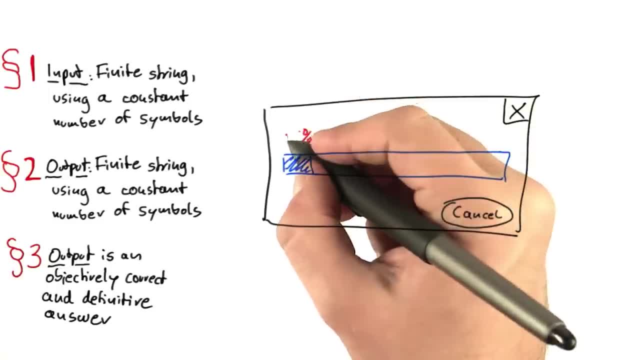 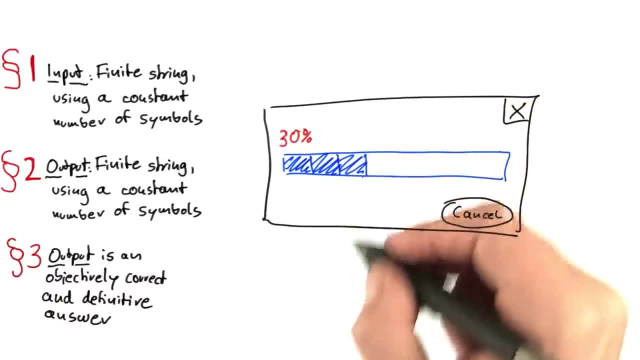 type of calculation or task on the computer. the computer tells you: yes, I'm 10% done. Then after a while this moves to 20%, after a while it moves to 30% And of course, Depending on what system you're working on, your mouse turns into this hourglass here. 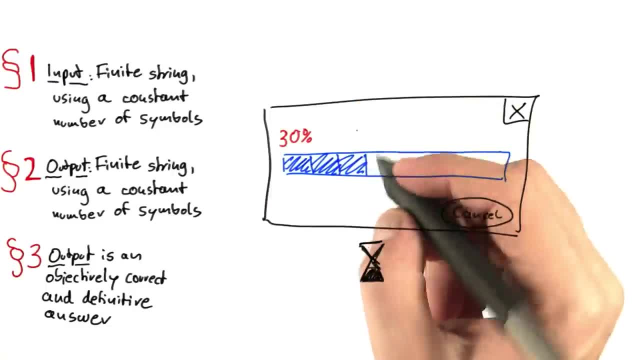 and now the progress bar gets stuck and it stays there. You go have lunch, you come back and it stays there. So the question is: at some point in time I mean you want this task to get done, but maybe in the next minute the computer will go on. 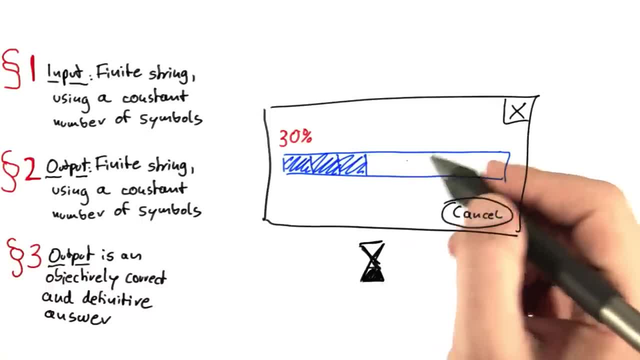 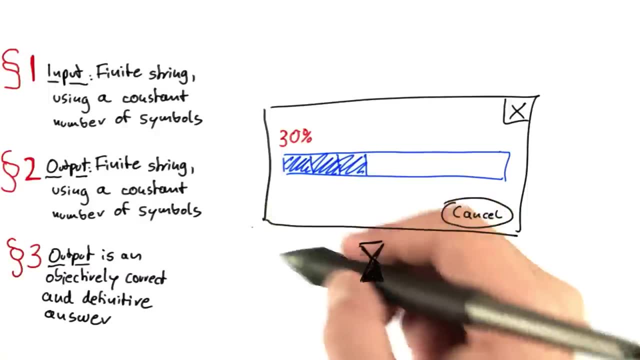 Maybe it's just thinking, it's just working, But it could of course also be that your program has crashed. If your computer stays that way for quite a time, well, you probably would assume that it has crashed, but you never know for sure. 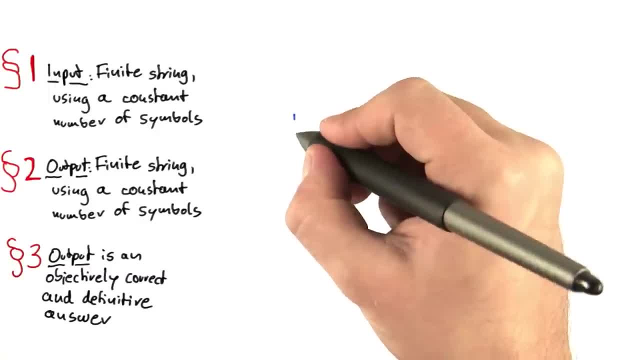 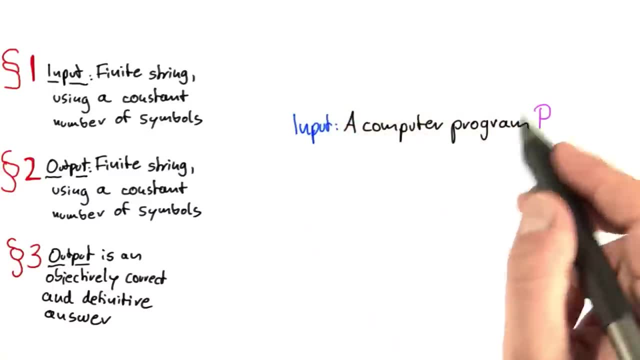 So what if we had an algorithm for that? What if we had an algorithm that took as input a computer program, P? It could be written in any language, basically so Python, C++, Java, whatnot, And of course we also want an input for that program. 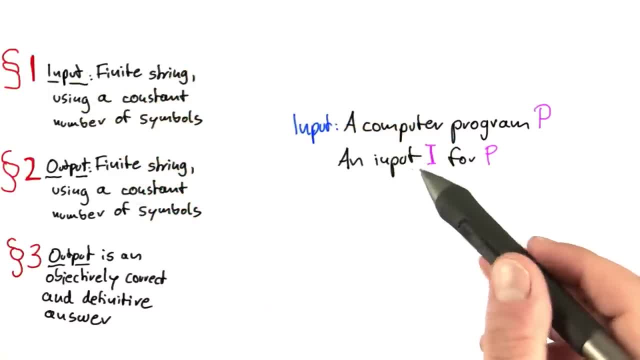 And the input, of course, in accordance with rule number one, will be a finite string using a constant number of symbols, And actually the program, of course, will be as well, So it may be, for example, the source code of a program.